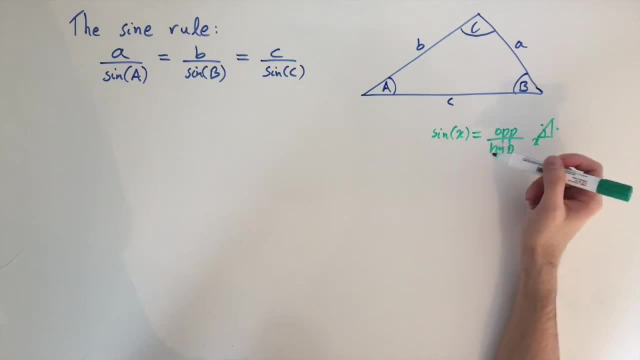 So this is the definition of sine. but to use sine we need a right angle triangle. so this has to be 90 degrees. So we want to find expressions for sine of a and sine of b, but to do that we need a right angle triangle. So we're going to use a little trick, we're going to drop down this line. 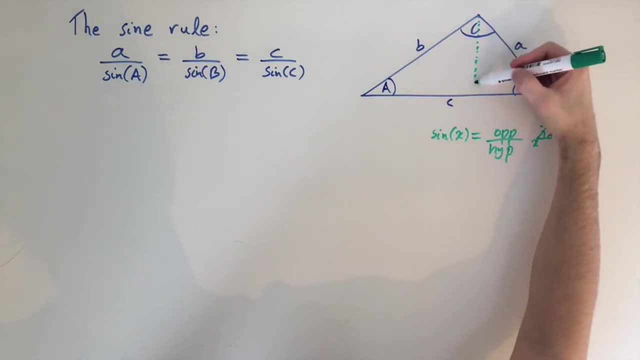 here. I'm going to drop down this line here, and we're going to drop down this line here and we're going to draw this dotted line all the way down. So we create two triangles, and these are both now right angle triangles, and I'm just going to label the length of this line h. So now we have a right. 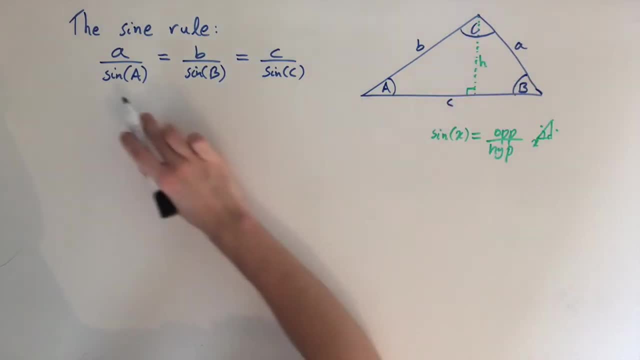 angle triangle with this angle a, which means we can write what sine of a is using this definition. So sine of the angle a is the ratio of the opposite side divided by the hypotenuse. So here the opposite side is this one which has a right angle triangle and this is the ratio of the. 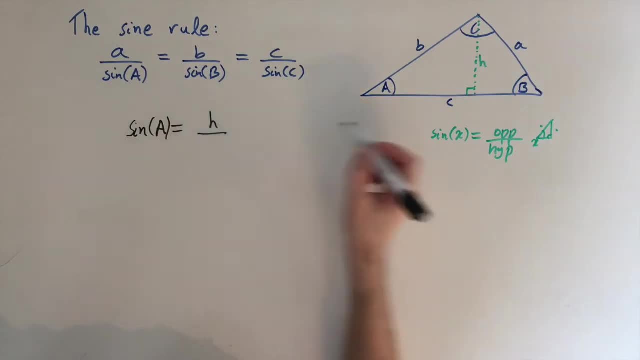 length, h. So we have h divided by the length of the hypotenuse, and the hypotenuse is the longest side. so it's this one, it's b. So sine of a equals h over b, and we don't know what h is, but what we. 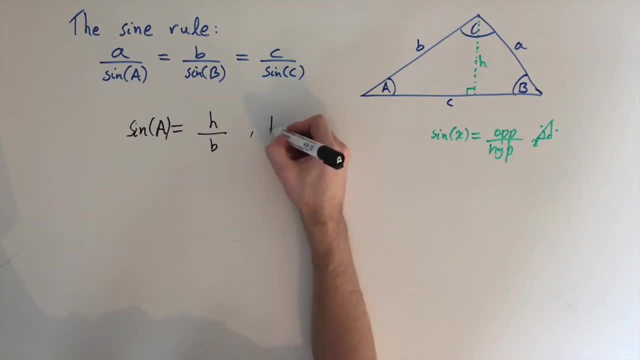 can do is we can rearrange again in terms of h. So I'm just going to bring up the b and we have: h equals b times sine of a, and our plan is to find another expression for b sine of b, and then we can eliminate h. 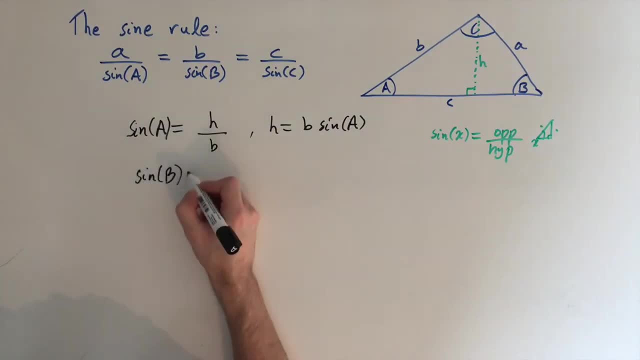 So to find sine of b. it's kind of a similar strategy. We now look at this right angle triangle, the one on the right. So this is also 90 degrees and we can just use this definition. So the ratio of the opposite length to the hypotenuse, the opposite is again h, but now the hypotenuse. 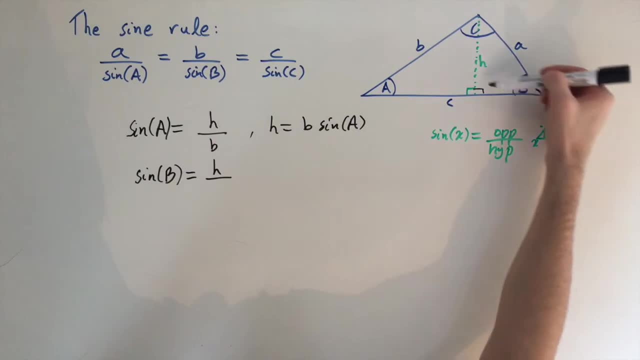 isn't b, it's actually this length, the longest side of the small triangle, and this is a. So we have h divided by a and again we can rearrange again in terms of h. So h equals a times sine of b. and this is really nice because we have two equations for h and so we can equate them, because